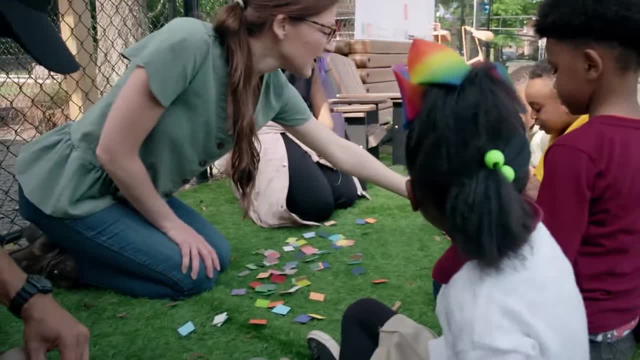 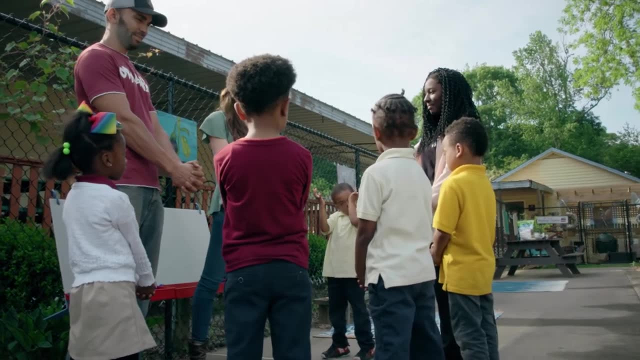 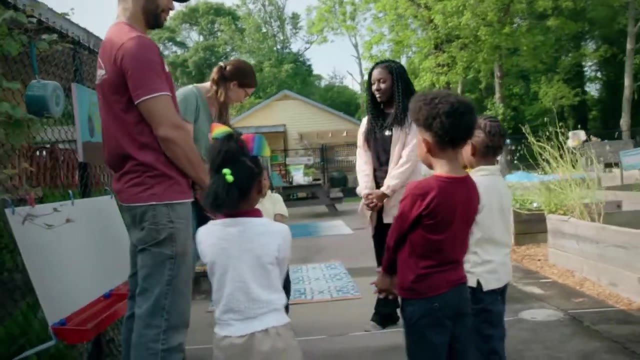 An outdoor activity can be started with an outdoor observation together. First sit or stand with all of the students in a circle in an open place outdoors, Ask the students what is the same and what is different from our last visit to this space, And then give the children a few silent seconds to just listen and look to the world around them. 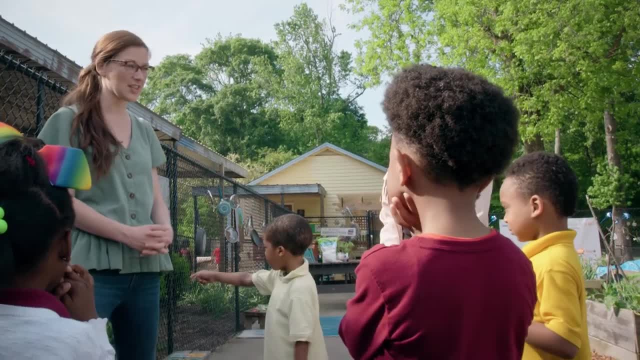 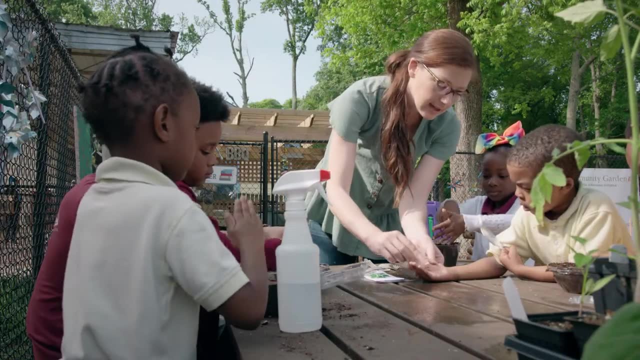 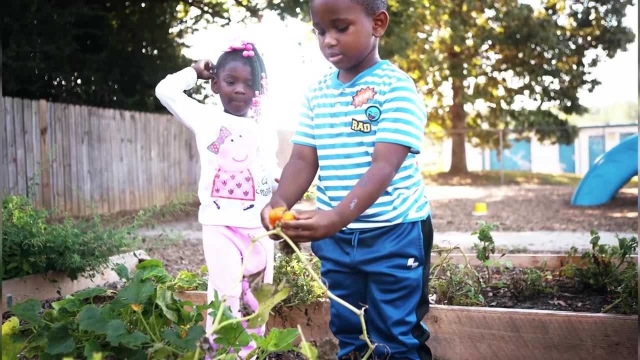 Following that time provide time for the children to share what they observed. There are many outdoor activities for every age level that can be done in the garden with minimal materials or planning. Mathematic Cognitive Development: Children can use size words to describe things found in the garden. 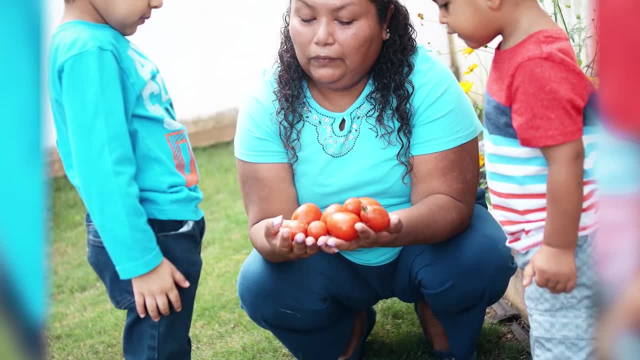 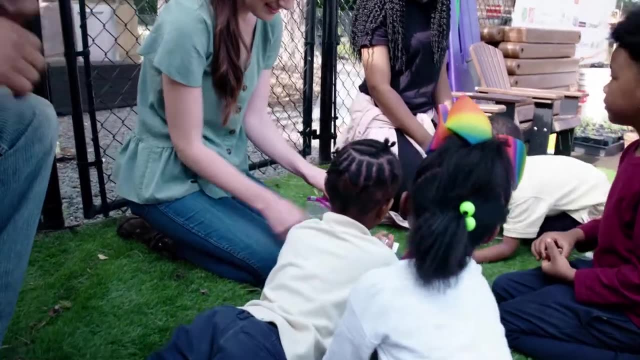 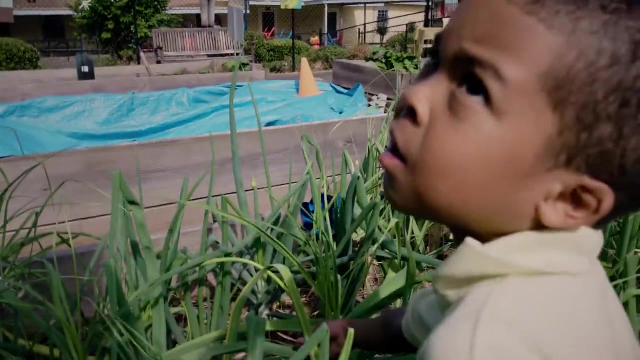 They can find objects of different shapes in the garden. Children can count the number of worms found in the garden or sort fallen leaves by color, shape or size. Science, Cognitive Development: Young children can observe and explore with their senses: sight, touch and smell. 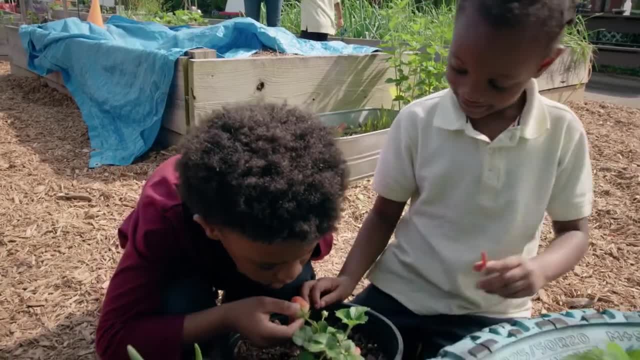 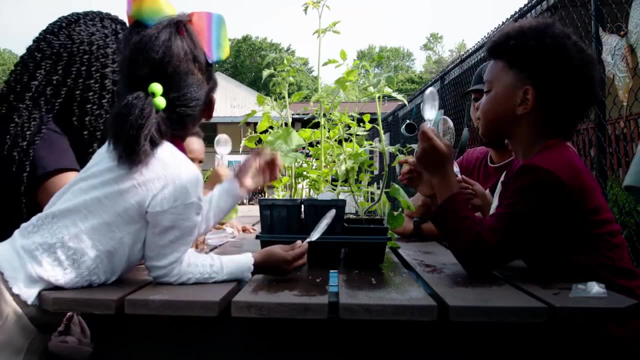 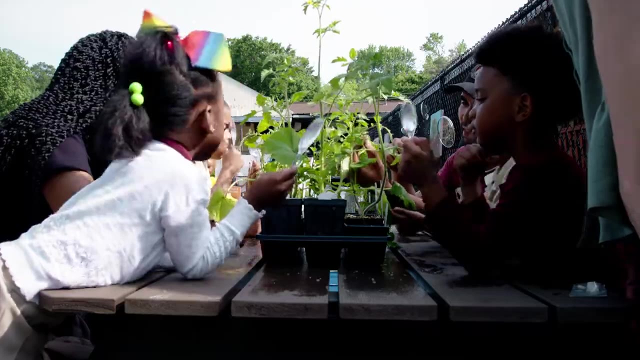 Children can show curiosity about the garden. Children can use a magnifying glass to look closer at things found in the garden. Children can record observations of plants and animals through drawings and dictation. Children can explore water, soil, sand and mud and build an understanding of what plants need. 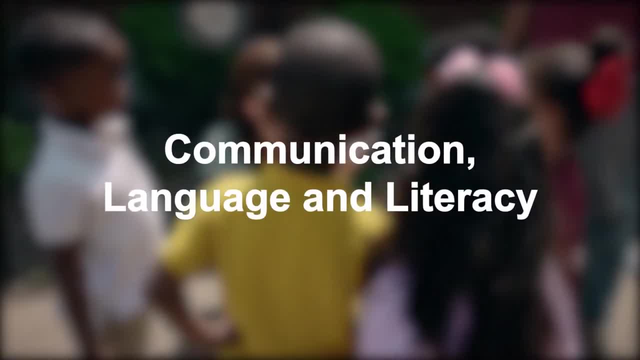 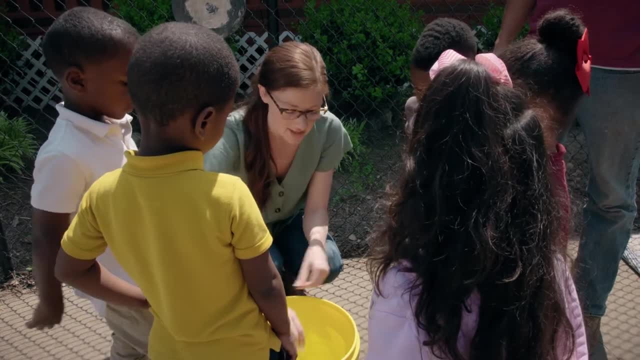 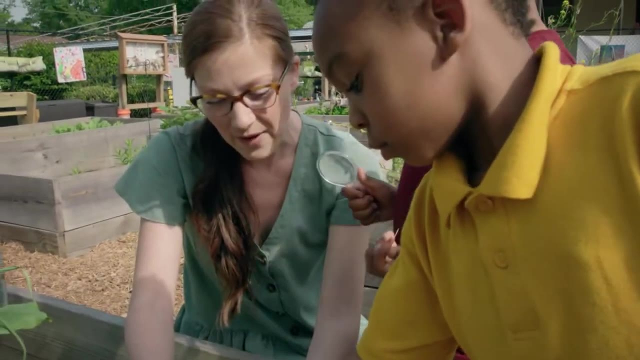 Communication, Language and Literacy In the garden. young children can listen to and follow simple directions for garden tasks. They can ask and answer questions about what is being observed in the garden. Children can describe the garden activities using expanded sentences and details. 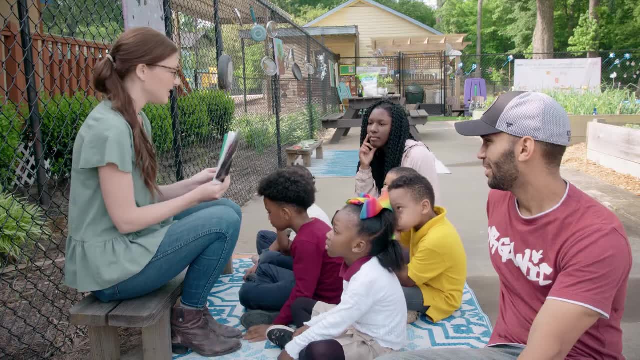 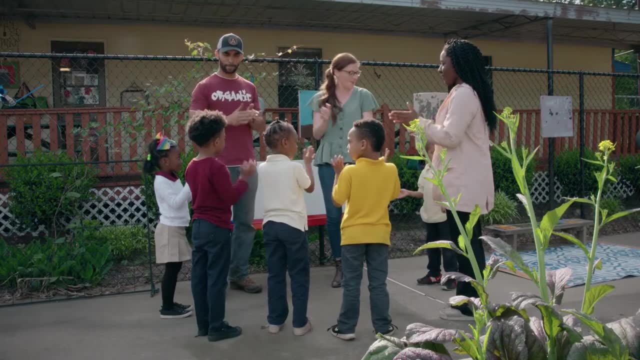 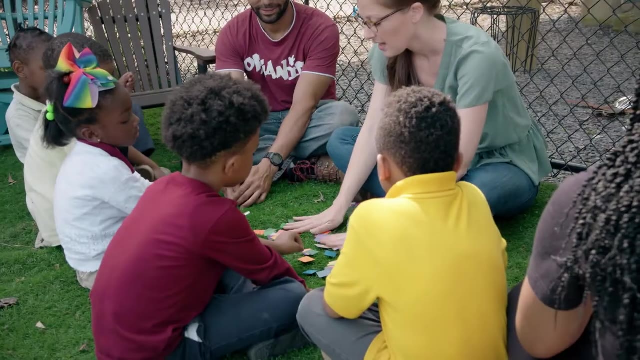 And children can build vocabulary through activities, books and conversations about the garden. Creative Development: Young children love to listen to rhymes, finger plays, songs and stories about the garden. Children can describe what colors are seen in the garden through the different seasons.